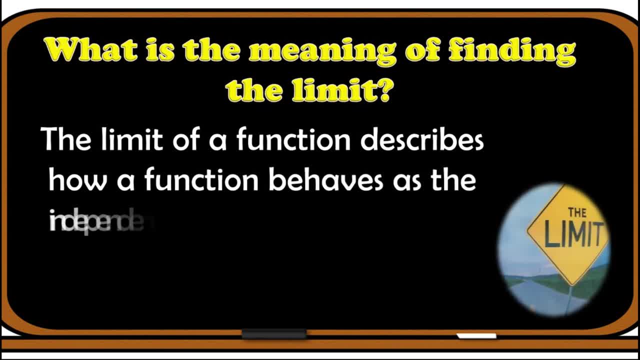 a function. describes how a function behaves as the independent variable x gets closer to a certain number, or is called a constant. Keep in mind that the variable can only take values very close to the constant, but it cannot be equal to the constant itself. The. 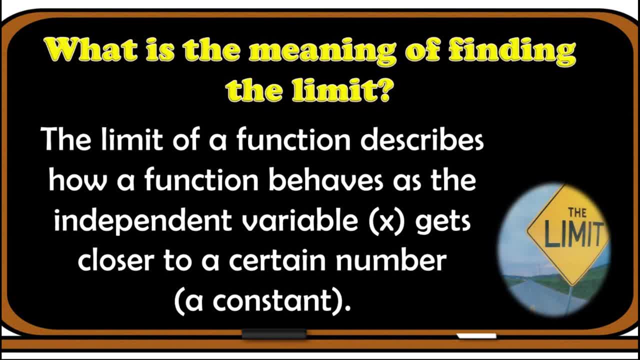 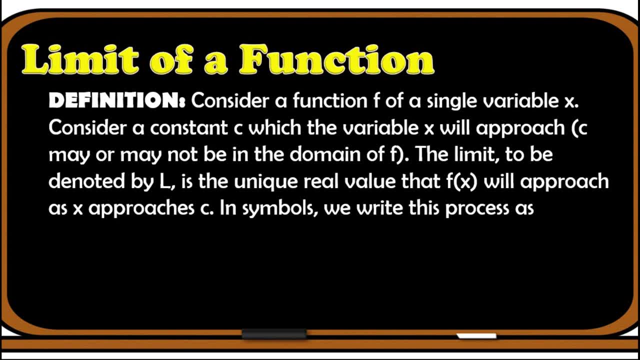 limit will describe what is happening to the function near the constant. Let us now define limit mathematically. Consider a function f of a single variable x. Consider a constant c which the variable x will approach, and c may or may not be in the domain of f, The limit to be denoted by. 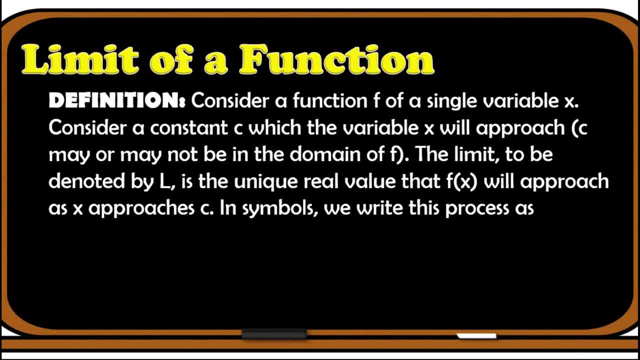 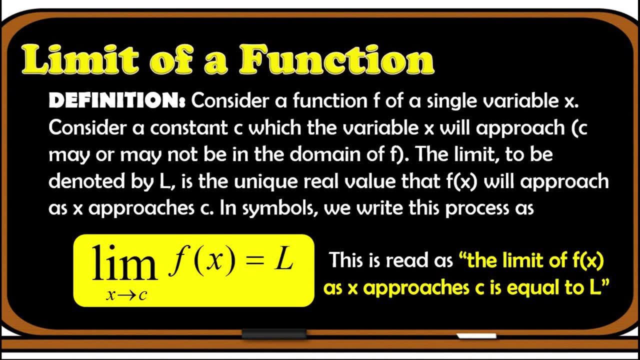 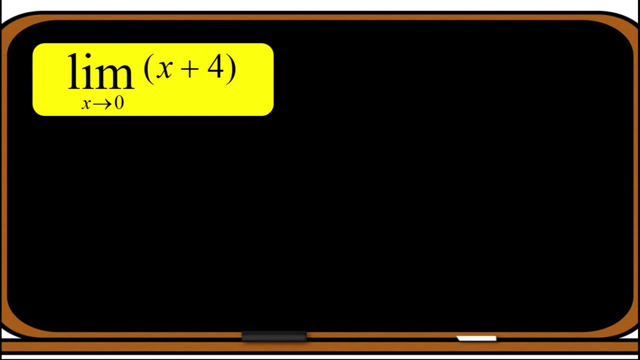 l is the unique real value that f will approach as x approaches c. In symbols we write this process as, which is being read as the limit of f as x approaches c. Consider this given problem: the limit of x plus 4 as x approaches 0.. The question here: 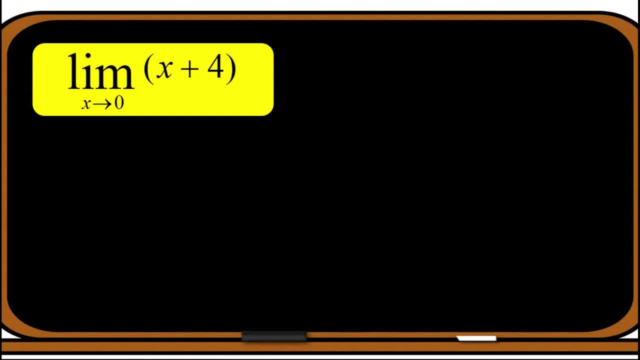 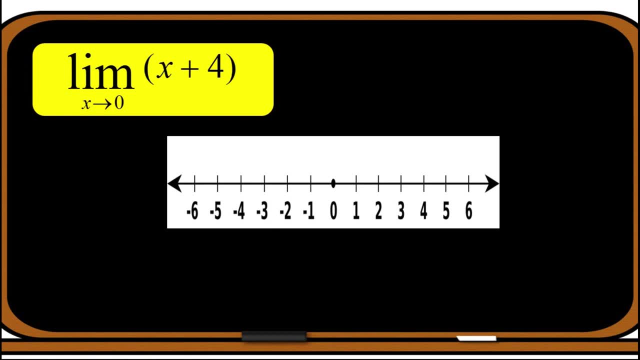 is: what value will the function approach to as the independent variable x approaches zero? If we have a number 9, there are 2 ways to approach zero. It can be through values on its left and through values on its right. Let us first consider approaching zero from. 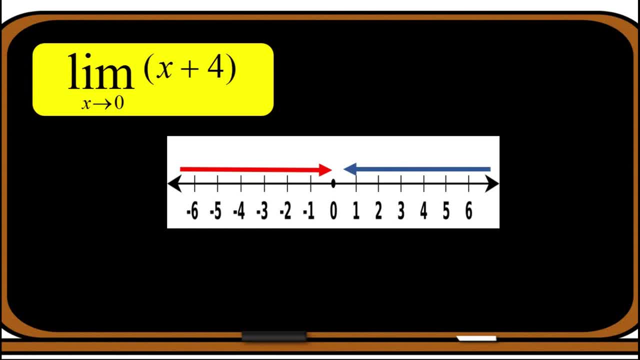 its left. Let us first consider approaching zero from its left. Let us consider approaching left or through values less than zero. the limit that we get from left going to zero is what we call the left-hand limit, and it is represented by the limit of f. 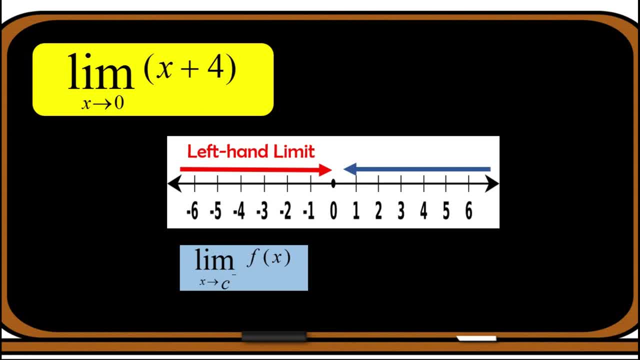 of X. as X approaches C from the left using the symbol negative and from the right, going to zero, it is called the right-hand limit. so we have this symbol. the limit of f of X. as X approaches C from the right using the symbol plus sign for the limit of the function X is the left-hand limit must have the same. 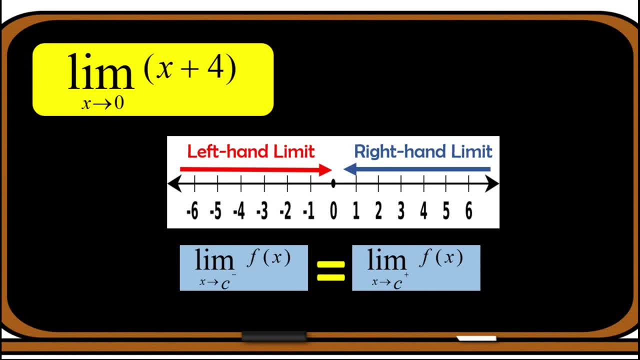 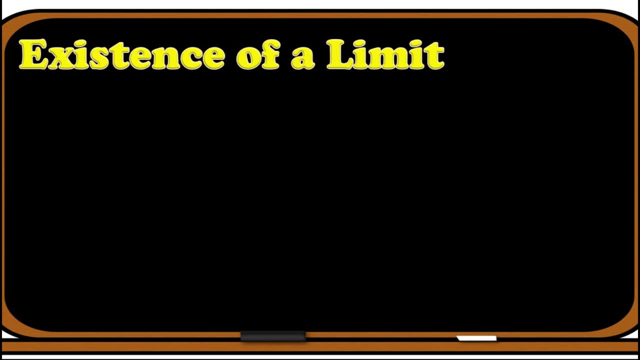 value with the right-hand limit. in other words, for a limit- L- to exist, the limits from the left and from the right must both exist and be equal to the value of L. let's talk about the existence of a limit. the question is: this limit always exists? 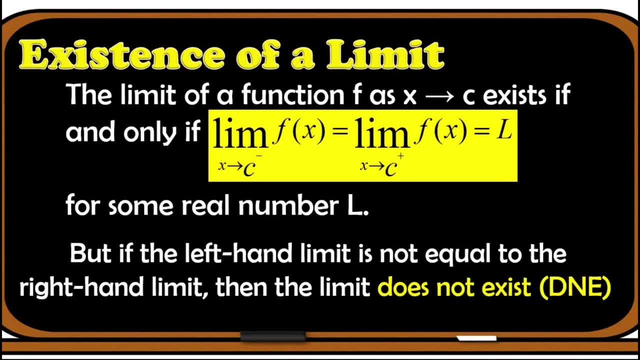 the limit of a function, f, as X approaches C, exists if, and only if, the left-hand limit is equal to the right-hand limit for some real number, L. but if the left-hand limit is not equal to the right-hand limit, then the limit does not exist. or if one of this does not exist, automatically the limit does. 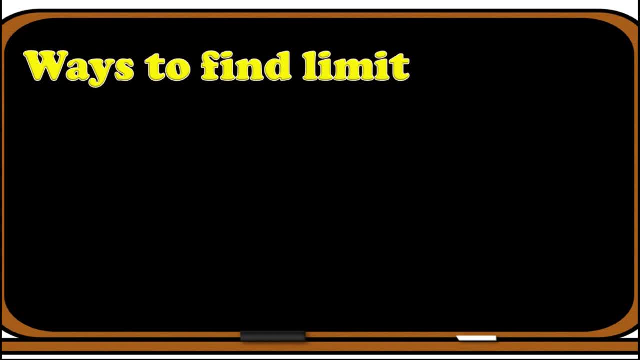 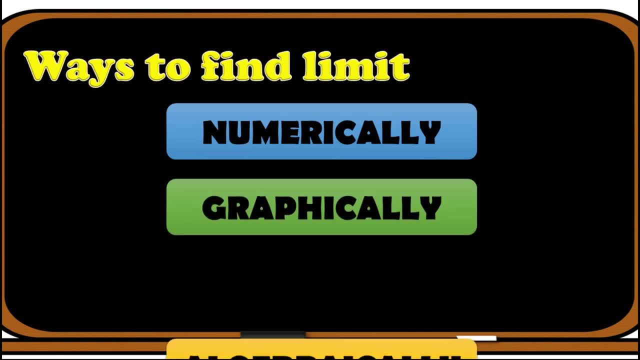 not exist as well. how do we find the limit? here are the following ways. first, we can find the limit of a function, f as X approaches C from the left, using the symbol. we can do the numerical method, or numerically, second, graphically and third, algebraically. 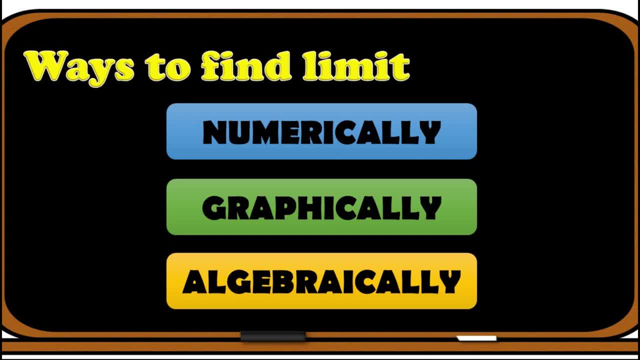 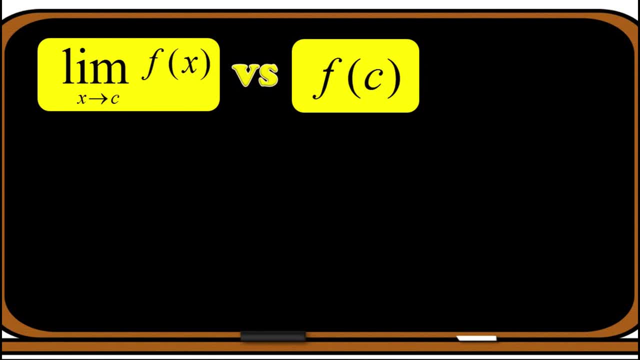 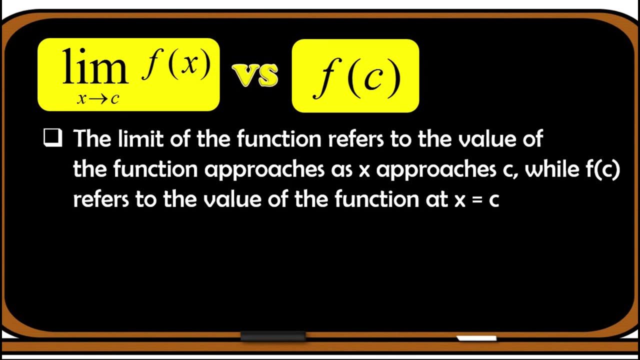 in the next videos we are going to discuss each of these methods. this time let us talk about the difference of the limit of a function as X approaches C and f of C. when we see limit of the function, it refers to the value of the function approaches as X approaches C. when we say f of C, it 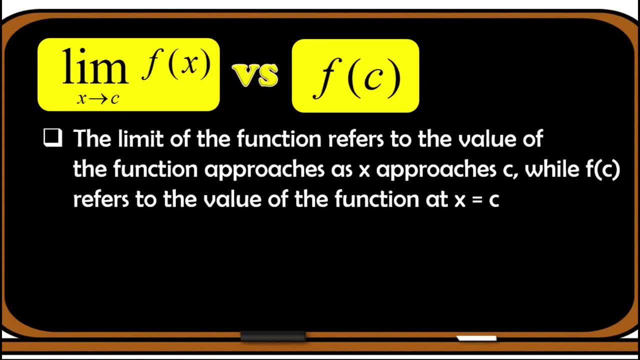 refers to the value of the function at. X equals C in limits. it is very important to understand that this tool may have the same or different values. sometimes both of them exist, or both of them do not exist, or only one of them exists. it must be clear that the exclusion of a value from 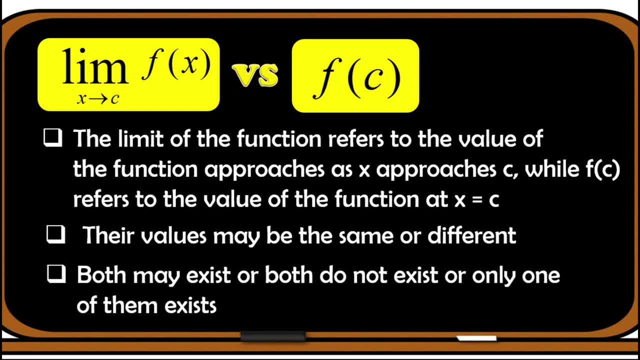 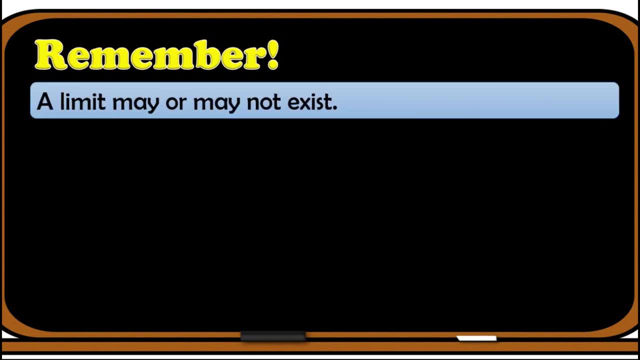 the domain of a function does not prohibit the evaluation of the limit of that function at that excluded value, provided, of course, that f is defined at the points near the value of C. what are the important things that you need to take note? first, a limit may or may not exist. 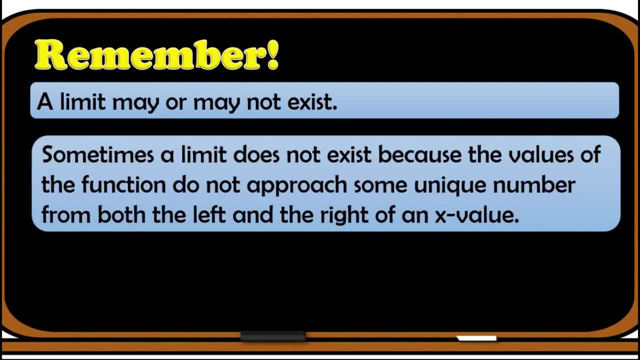 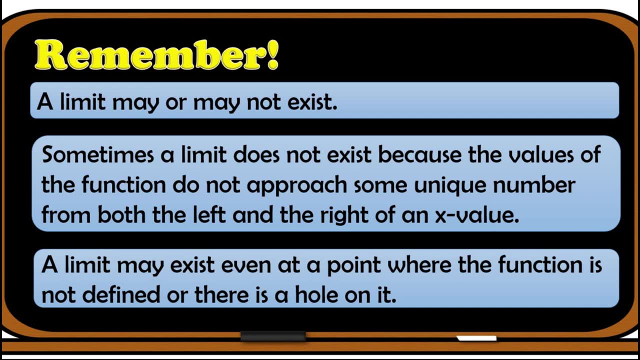 sometimes a limit does not exist because the values of the function do not approach some unique number from both the left and the right of an x value. third, a limit may exist even at a point where the function is not defined or there is a hole on it, since limits indicate.